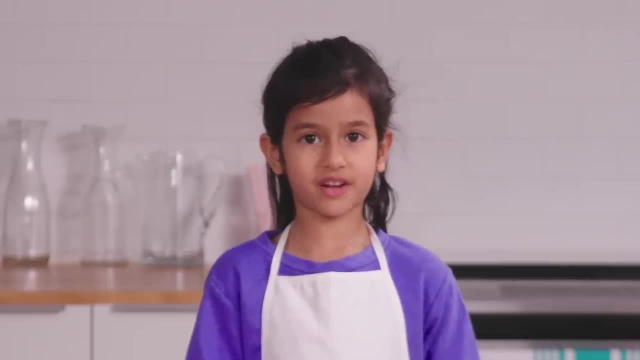 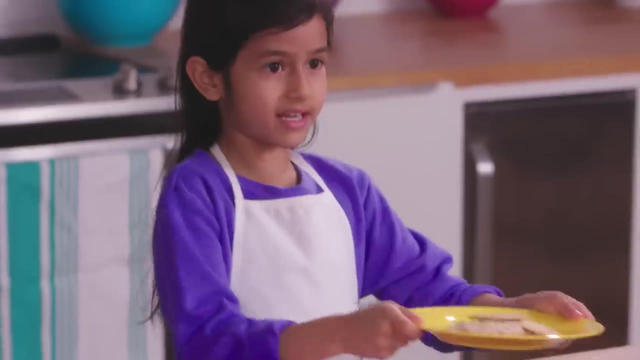 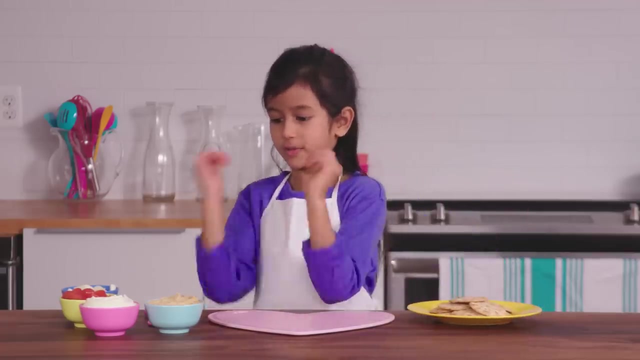 Today I'm going to teach you how to make some of my favorite healthy snacks from Butterbean's Cafe. Let's make tomato cheese crackers. First, we need crackers. You can use whole grain or gluten-free. Next, we'll need hummus or cream cheese. 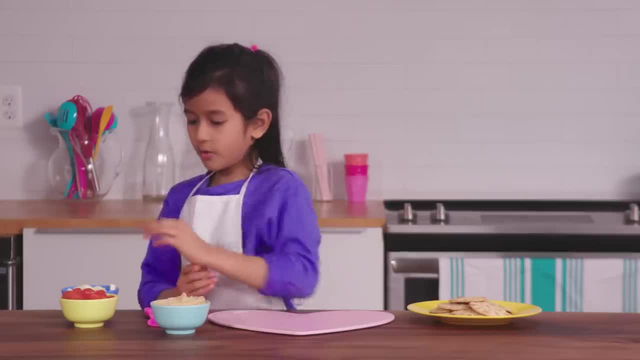 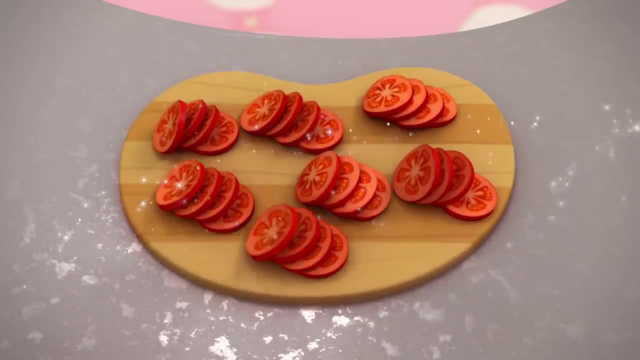 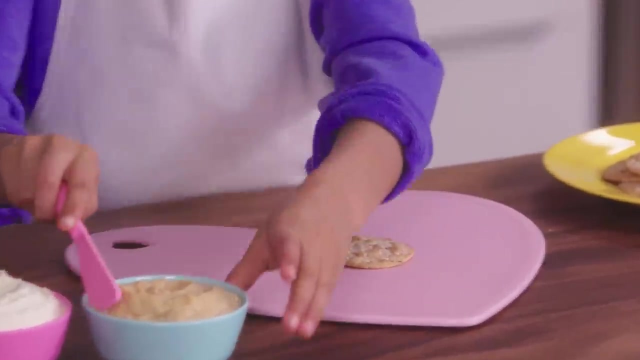 Today I will be working with hummus. Now we need some cherry tomatoes and mozzarella sticks cut into halves. Let's get started now. First we need one cracker, Then we spread the hummus or cream cheese along the top. 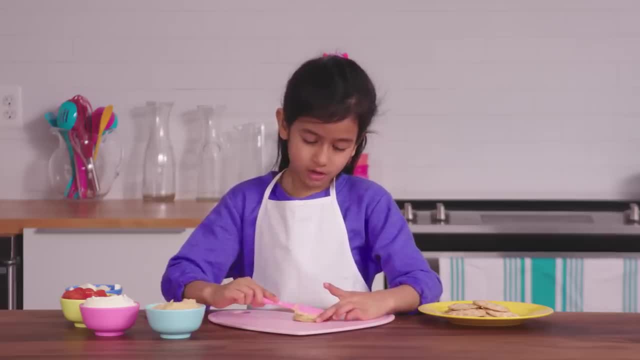 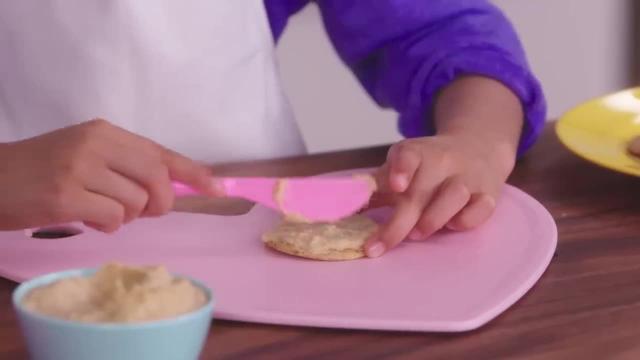 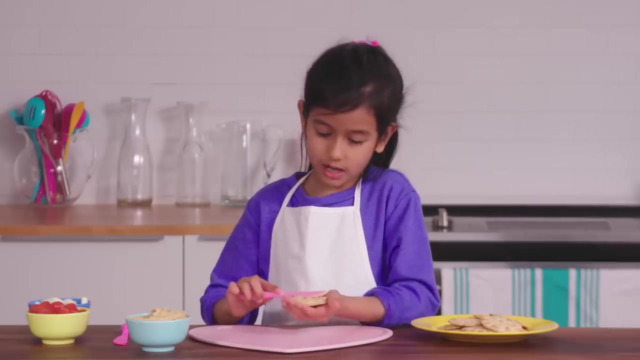 I'll give you a tip. If you're using cream cheese, it'll be a bit hard to spread it. You might have some mishaps. Yikes. If you're using hummus. I have another tip: Don't add too much, because then it'll get all over your hands. 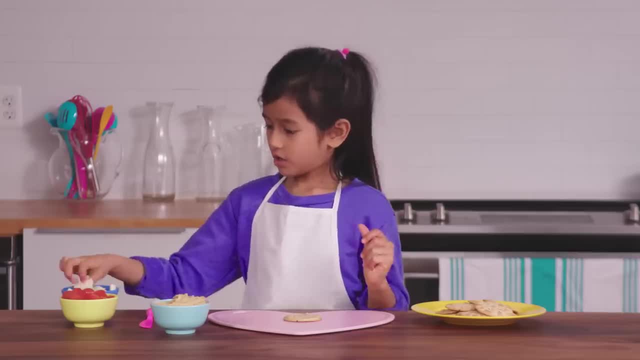 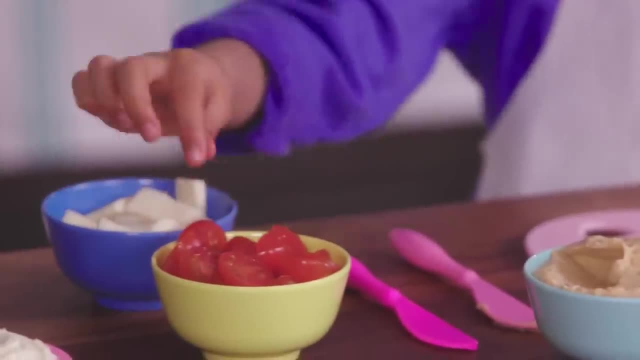 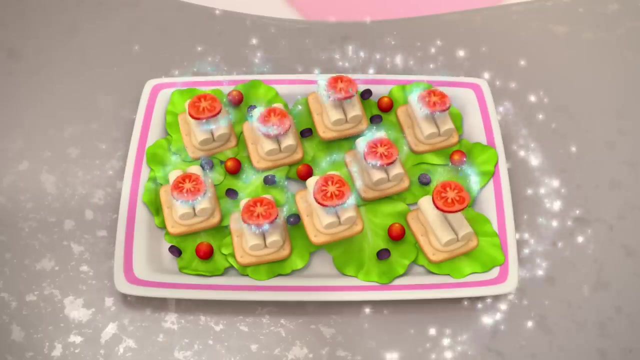 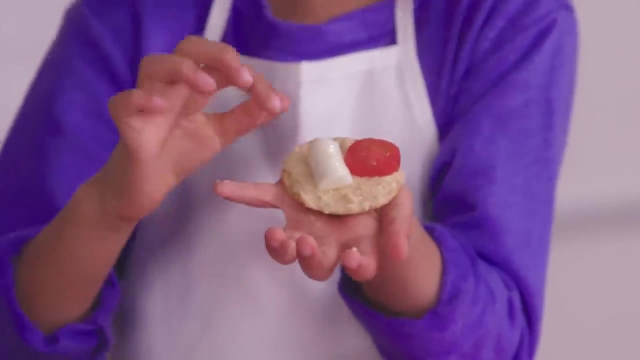 And you don't want that to happen. right Now, we place a mozzarella stick on the cracker. Next we'll need one cherry tomato half. Does this remind you of anything? Because it reminds me of the number 10.. 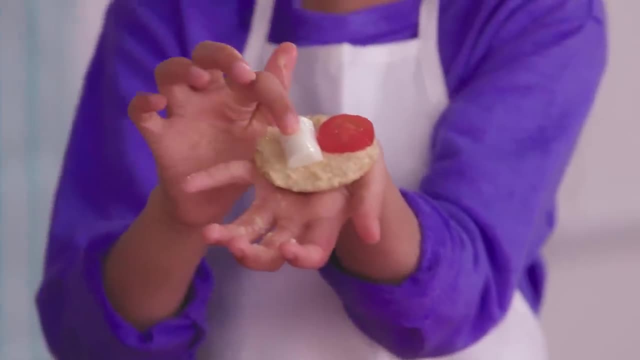 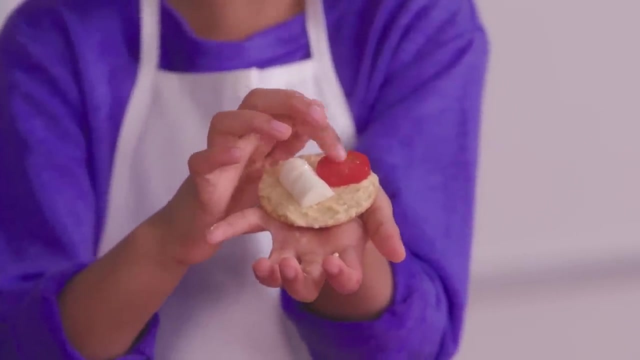 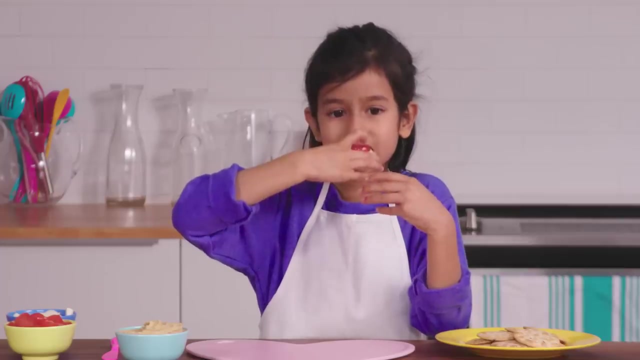 Because the mozzarella stick is the number 1 and the cherry tomato is the number 0.. Mmm, looks great, doesn't it? Now for the fairy finish. Wow, thanks, Butterbean Mmm. Hi, I'm Kid Chef Josiah. 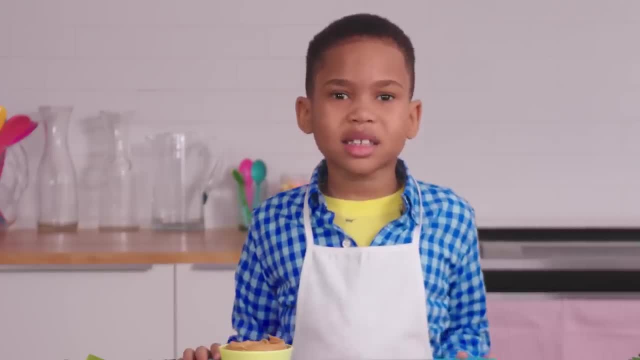 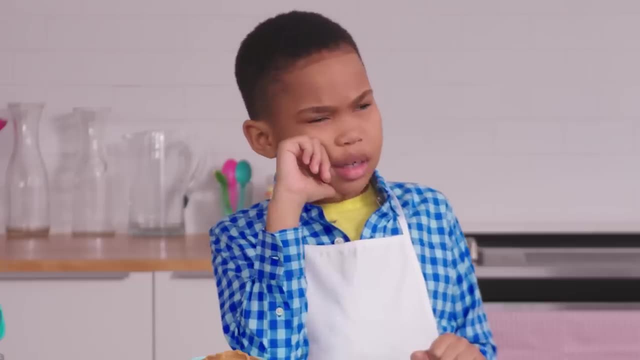 And today I'm going to be teaching you how to make one of my favorite healthy snacks from Butterbean's Cafe. Let's make ants on a log. So, first things first, we need a log and some ants. Just kidding, We'll use these celery sticks, some peanut butter and some raisins. 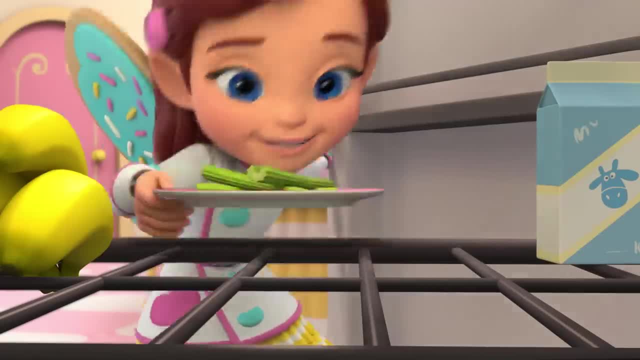 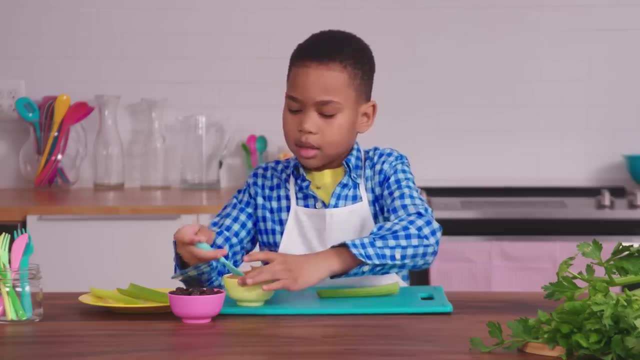 So first we take a celery stick, Sit it down, Then you put some peanut butter along the top, And then you, beautiful, duck, And you put some peanut butter around it, And you put some peanut butter around it.